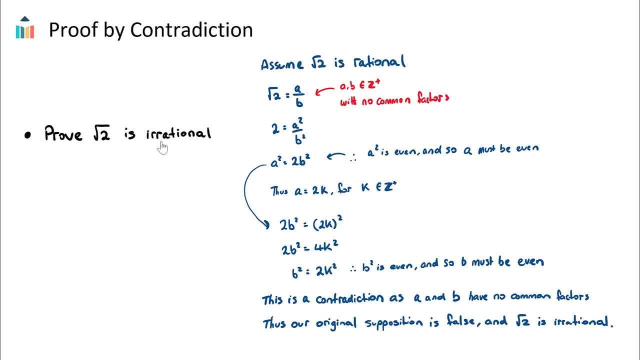 opposite and show that that isn't correct. We want to assume the negation, which is another word for the opposite of our conclusion. show that that isn't actually correct or show that it is false, so that we can say our original conclusion must be true. Okay, so that's the basic idea of proving something by 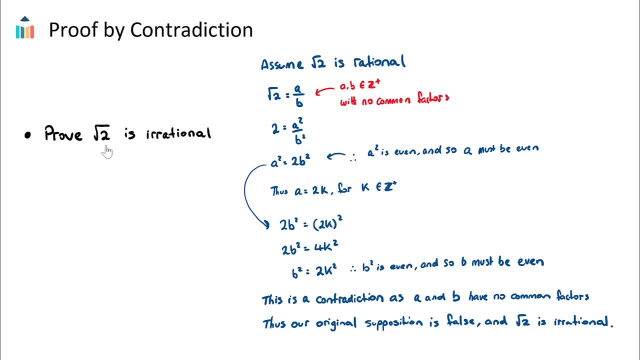 contradiction. Okay, so let's go through the steps. If we want to prove that root 2 is irrational, let's take the opposite stance here. Let's start with the opposite of the conclusion. Let's assume root 2 is rational. Now, if root 2 is, 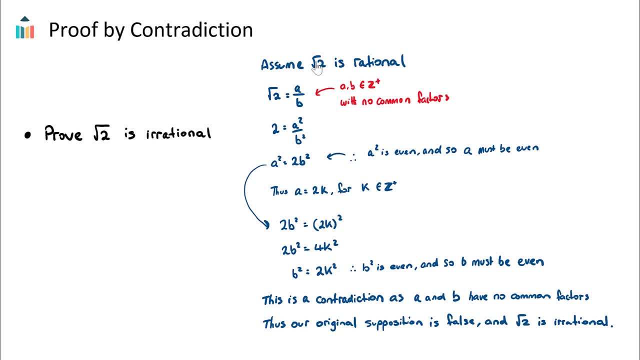 rational. well, what's a rational number? A rational number is something that can be expressed as a fraction. Let's say a over b and root 2 is clearly a positive number here. so we are going to say that a over b, where a and b are both positive integers, and that a and b 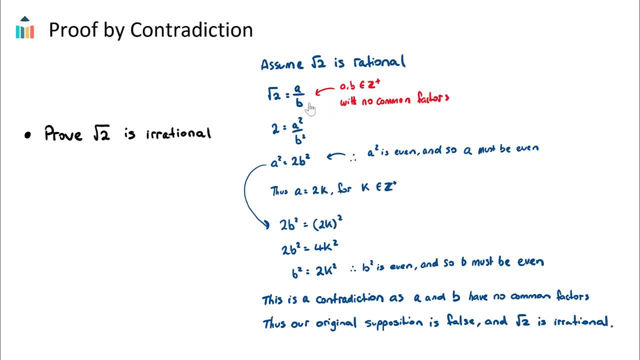 are in, they have no common factors. This is in its most simple form. Okay, so this is assuming that root 2 is irrational by expressing it as a over b, and it's very important here that a and b must have no common factors. Okay, so what we can do is 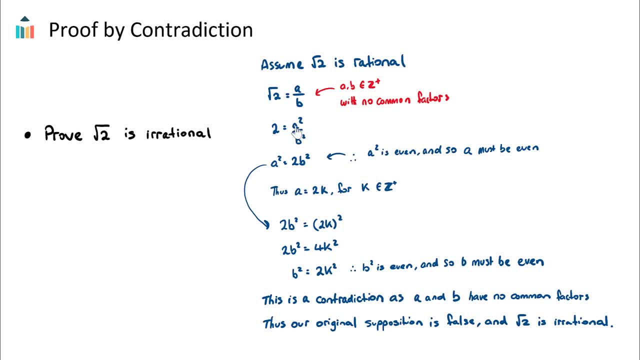 square both sides and therefore we will get: 2 is equal to a squared over b squared. I can multiply both sides by b squared and therefore I'll be left with a squared equaling 2 times b squared. Now at this step here we can say: well, if a squared is equal, 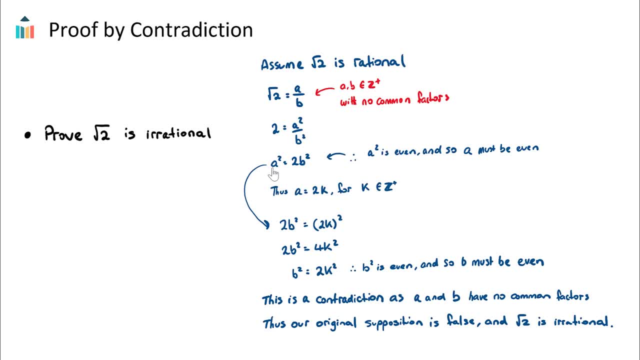 to 2 times b squared. well then, clearly a squared is even, because 2 times anything will give us an even number. So therefore, we can say: a squared is even. and if we know that a squared is even, what we therefore know is that a must be even, And you can confirm. 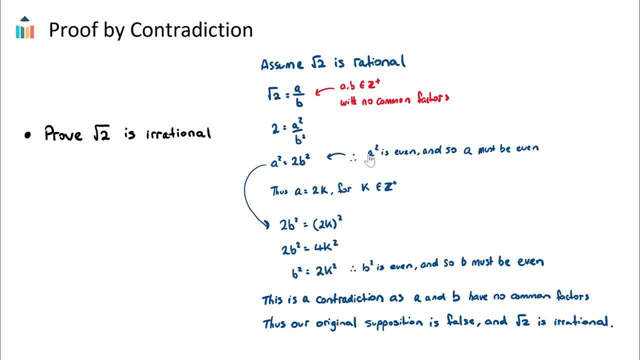 that If any squared number is even, the square root of that is equal to a squared. So we can say that the square root of that number will also be even. So we have concluded here that a must be even as well. So if we know that a is even, we can say that a is equal. 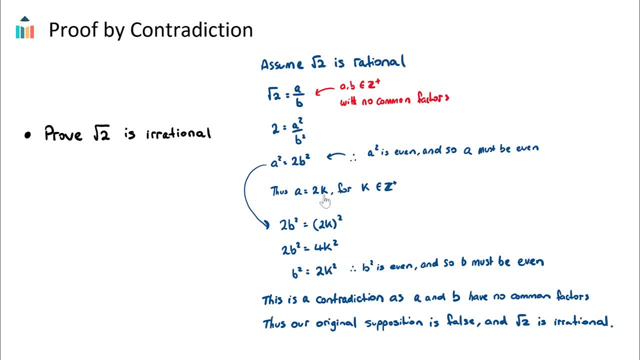 to 2 times k. Now, I've just introduced k here as a variable, but if k is any positive integer, well, 2 times k will represent any even number. Okay, so a can be expressed as 2 times k, And what we can therefore do is rewrite this one here and say: well, 2b squared.